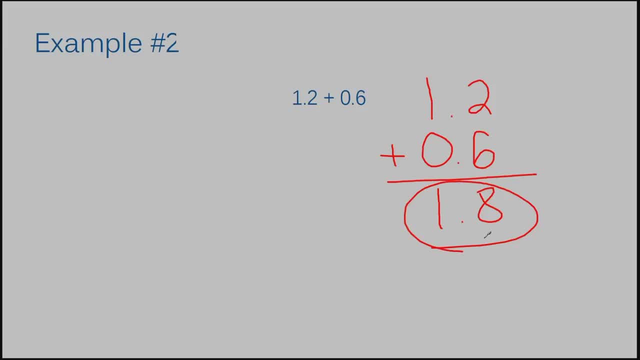 Let's move on to example number two. Example number two. We have five and twenty-one hundredths and three and twenty-five thousands. Again, I'm just adding numbers and subtracting. Again, I'm going to line the numbers up, stacking the decimals directly on top of each other. 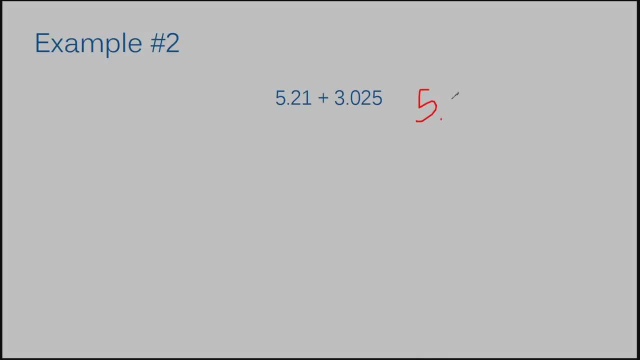 5 and 21 hundredths. And then I have 3. 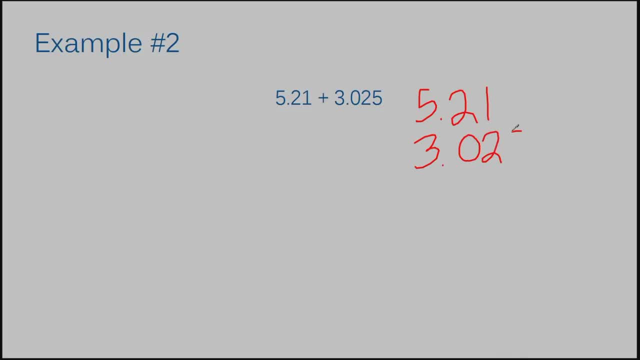 Write my 0, 2, 5, and 25 thousandths. I'm going to write my addition sign and draw my line. For this example, because our numbers don't have the same amount of digits, I'm going to fill in this top number with an extra 0. This 0 is acting as a placeholder and it's going to help me make sure I keep my numbers lined up. 0 plus 5 is 5. 1 plus 2 is 3. 2 plus 0 is 2. Bring down my decimal. 5 plus 3 is 8. 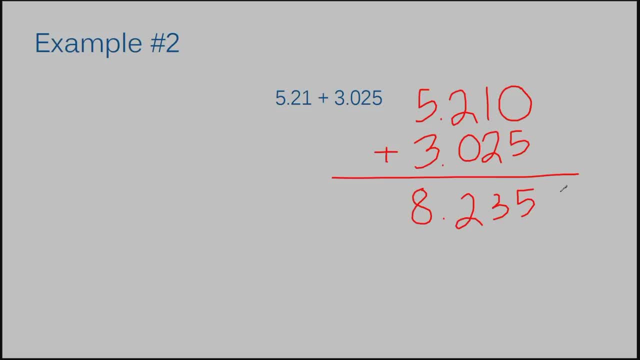 The answer to example number 2 is 8 and 235 thousandths. 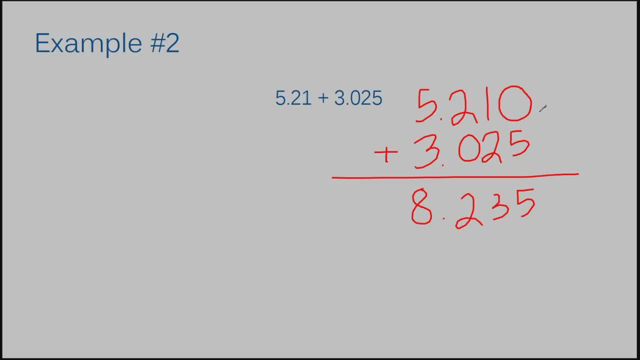 After we've filled in our 0 into the empty space, it made adding very simple. It's just like a regular addition problem. Let's move on to example number 3. Example number 3. I have 24 and 7 hundredths. 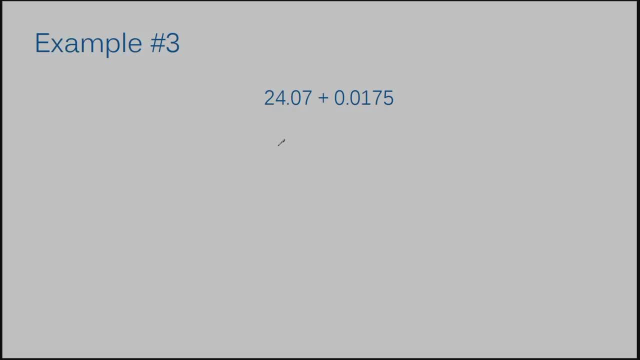 And I'm adding it to 1. 1 hundred seventy-five ten thousandths. 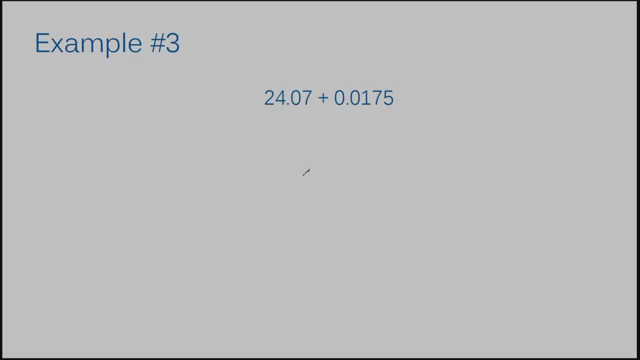 I'm going to start off by stacking the numbers directly on top of each other, considering the place value, like I've done before. 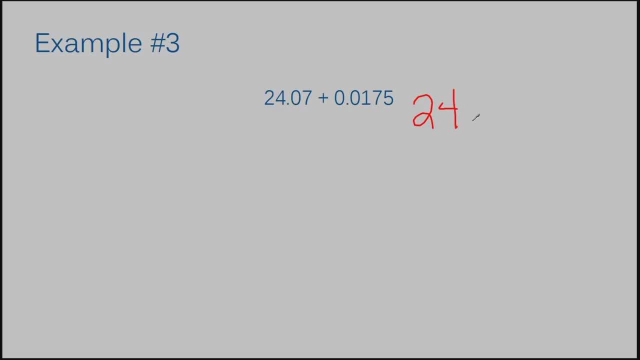 I have 24 and 7 hundredths. My 0 goes here this time instead of directly under the 2 because this 0 is written in the 1's place. The decimals need to be lined up. So I know that I should only start one space in. The 0 here and the 4 here are both in the same position. So they should be lined up on top of each other. Not the 0 put under the 2. The 2 is in the 10's place. Both the 4 and the 0 are in the 1's place. 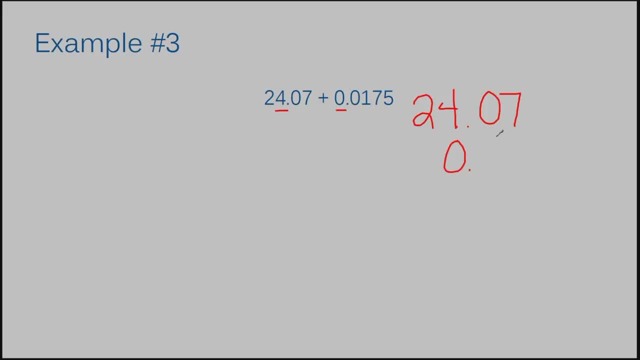 I'm going to write my decimal in. Now I'm going to fill in the rest of my number. 0 1 7 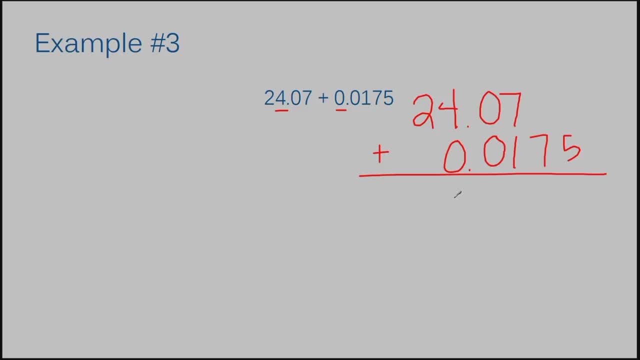 For this example, I have more than one place that is missing a number. So I'm going to fill in a 0 for all of those places. I'm putting in a 0 here and two 0's here. 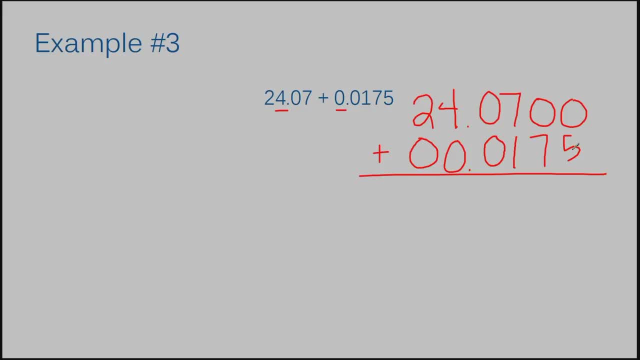 Now I'm going to add like normal. 0 plus 5 is 5. 0 plus 7 is 7. 7 plus 1 is 8. 0 plus 0 is 0. Bring my decimal straight down. 4 plus 0 is 4. And 2 plus 0 is 2. My answer to example number 3 is 24 and 875 ten thousandths. Let's move on to example number 4. 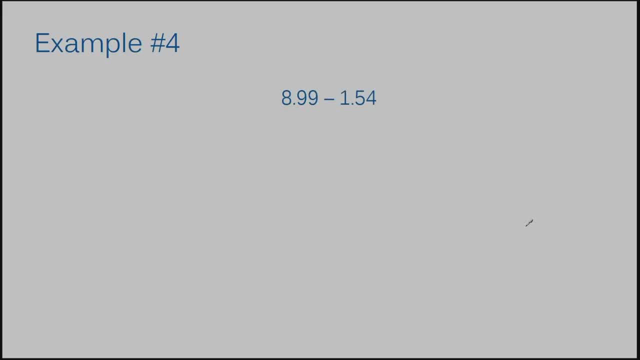 Example number 4. Example number 4. 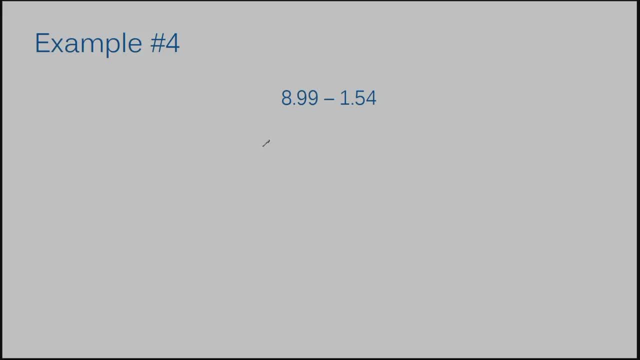 I have 899 hundredths and I'm subtracting this time. We're subtracting 1 and 54 hundredths. Again, we're going to line our numbers up by the place value. That means the decimals should be directly on top of each other. So I have 8 and 99. 1 hundredths. 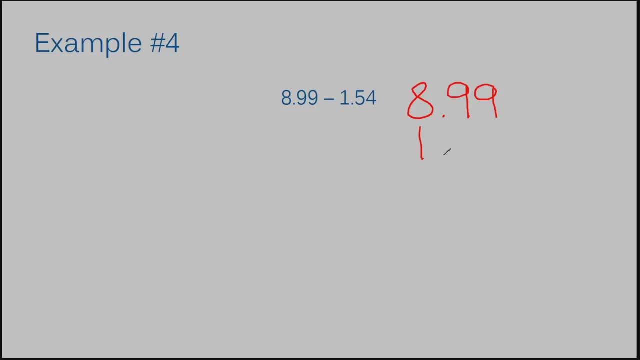 And I have 1 and 54 hundredths. I'm subtracting. 9 minus 4 is 5. 9 minus 5 is 4. Bring my decimal straight down. 8 minus 1 is 7. The answer to example number 4 is 7 and 4. Bring my decimal straight down. 9 minus 4 is 7. And 4 hundredths. 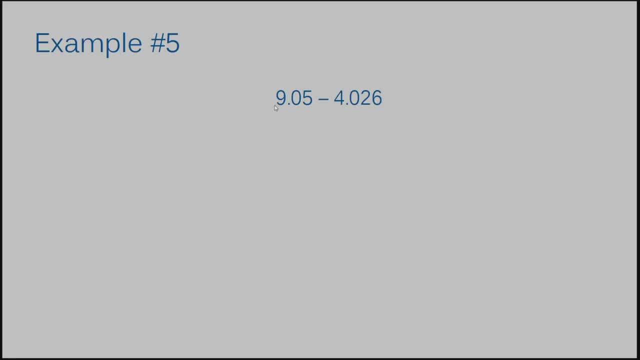 Let's move on to example number 5. Example number 5. 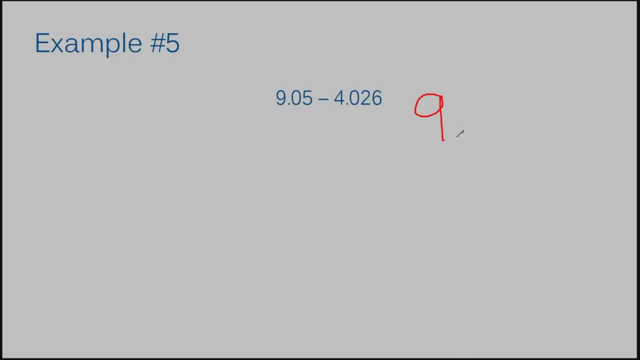 Again, we're stacking our numbers directly on top of each other. Again, we're stacking our numbers directly on top of each other. 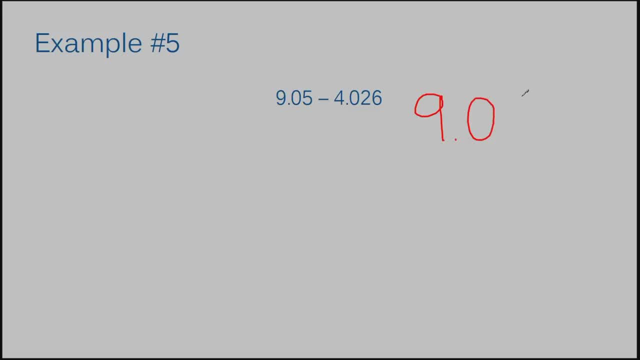 I have a 9. I have a 9. I have 5 hundredths. I have 5 hundredths. 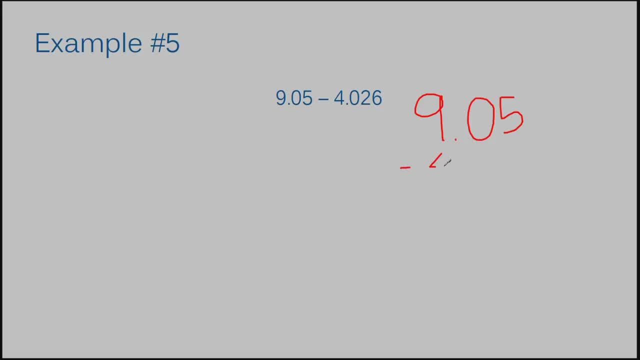 I'm going to subtract. I'm going to subtract. 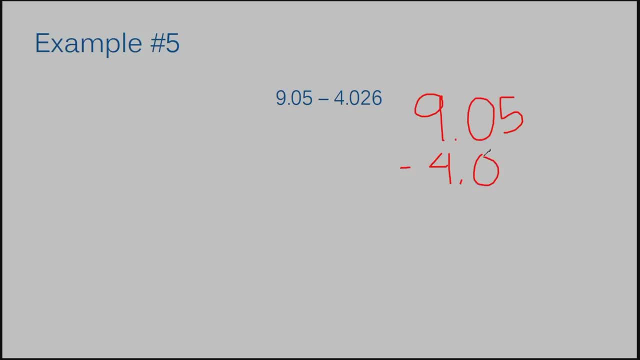 4. 4. And 26. 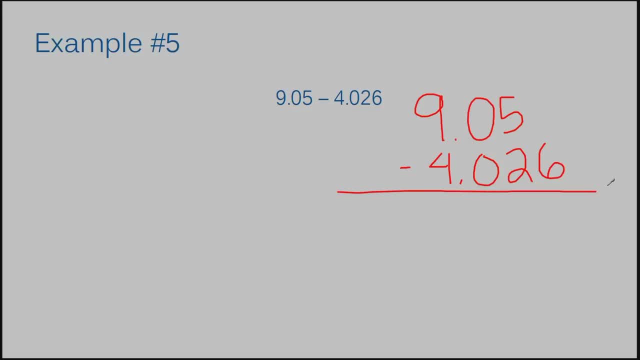 3 thousandths. Draw my line. 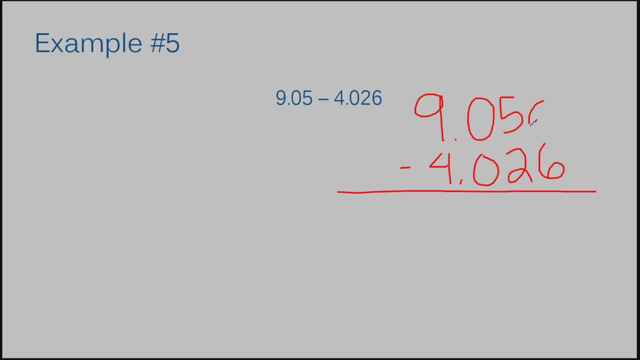 I need to fill in a 0 here. I need to fill in a 0 here. 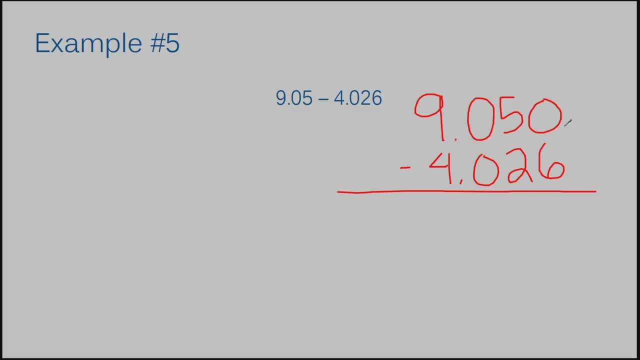 Again, we're subtracting. You need to know your rules for subtraction. 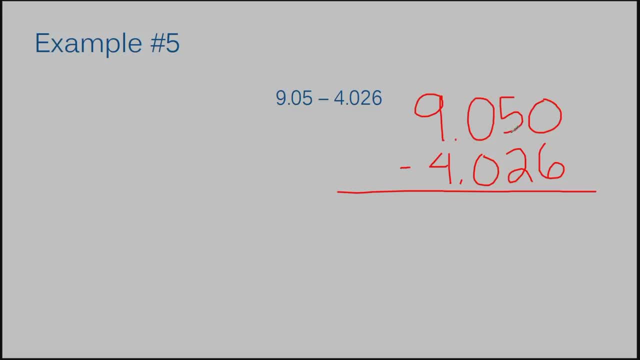 If you don't, go check out my subtraction video. 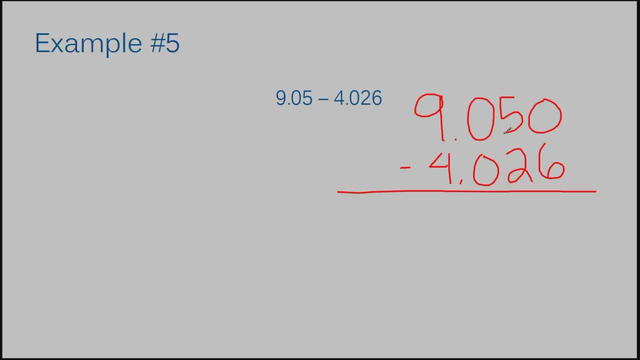 I have a subtraction of 2 and 3 digit numbers. I have a subtraction of 2 and 3 digit numbers. And I also have a subtraction with zeros video. And I also have a subtraction with zeros video. I can't take 6 from 0. 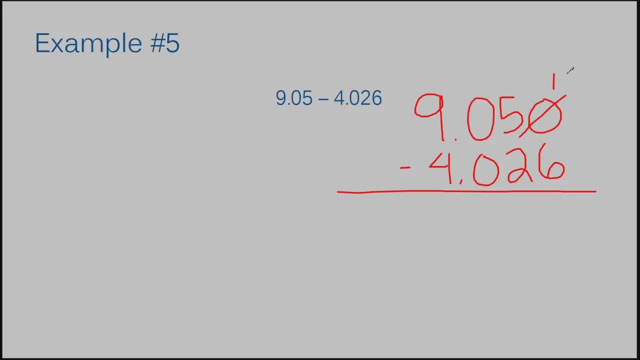 So I have to cross out this 0 and turn it into a 10. Now if I subtract here this becomes a 4. This becomes a 4. To make this number a 10 I had to borrow over here so the 5 becomes a 4. Now I can subtract here. 4 minus 2 is 2. 0 minus 0 is 0. 0 minus 0 is 0. Bring my decimal straight down. 9 minus 4 is 5. 9 minus 4 is 5. 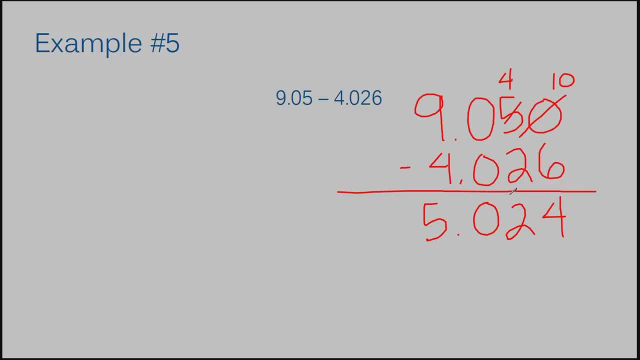 The answer to example number 5 is 5 and 24 thousandths. is 5 and 24 thousandths. is 5 and 24 thousandths. 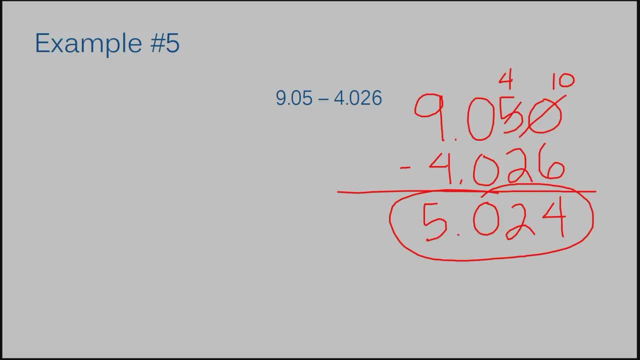 Let's move on to our final example. Example number 6. 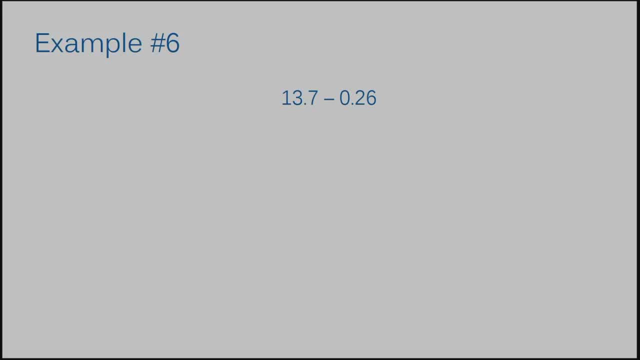 We have 13 and 7 tenths. We have 13 and 7 tenths. We have 13 and 7 tenths. 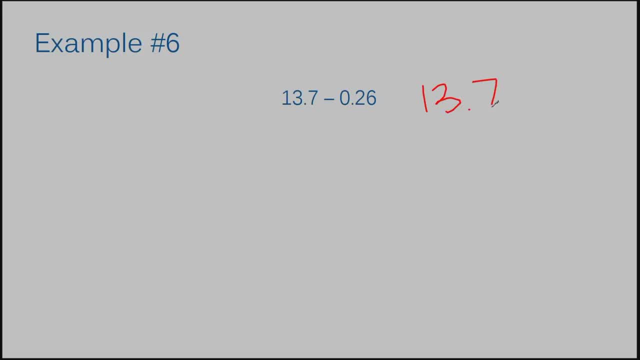 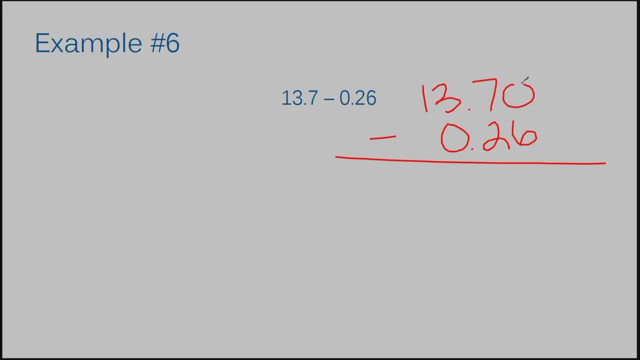 We're subtracting again. I need to fill in with zeros. I need to fill in with zeros. I can't take 6 from 0 so I need to cross out this 0 and turn it into a 10. 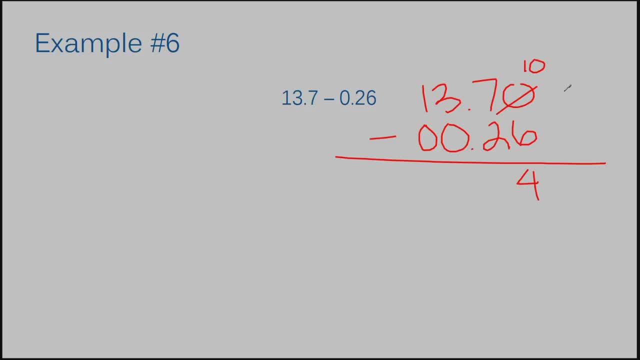 Now I can subtract this and I get 4. Now I can subtract this and I get 4. To make this a 10 I had to borrow from this 7 so it became a 6. 6 minus 2 is 4 also. 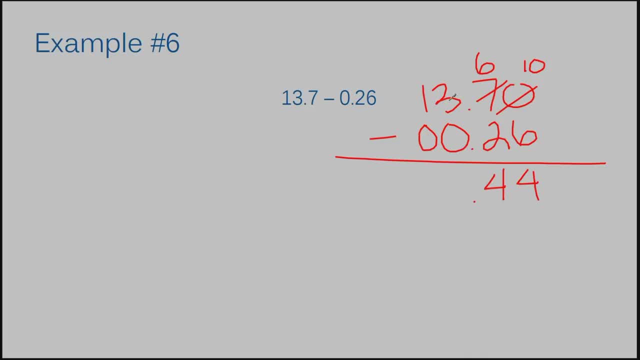 6 minus 2 is 4 also. Bring my decimal down. 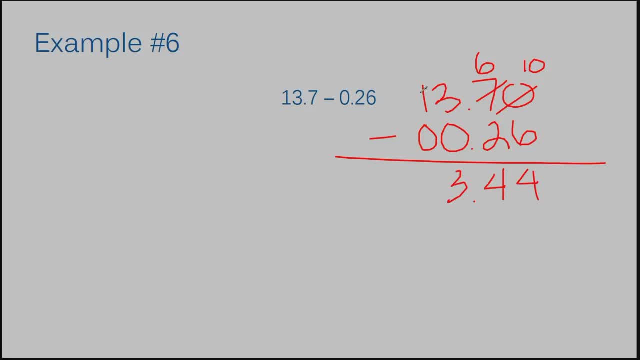 3 minus 0 is 3. 3 minus 0 is 3. 3 minus 0 is 1. 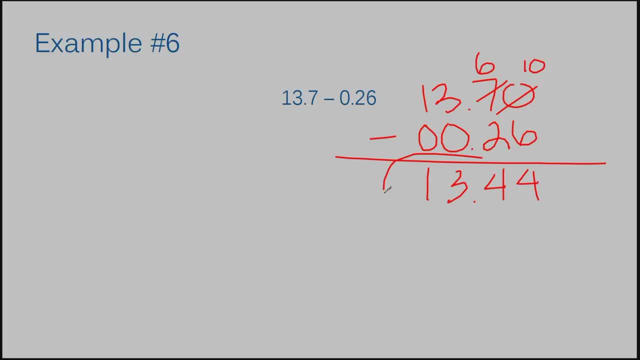 The answer to example number 6 is 13 and 44 hundredths. That's my last example. Thanks for watching! 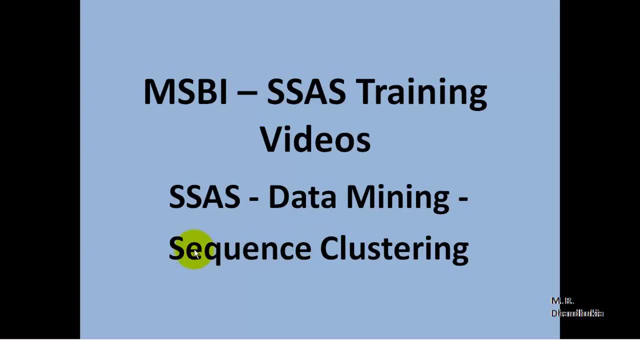 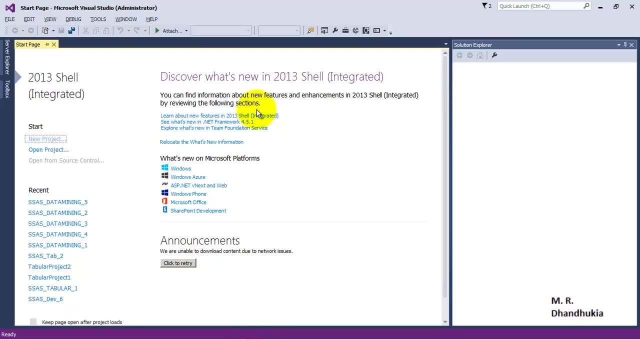 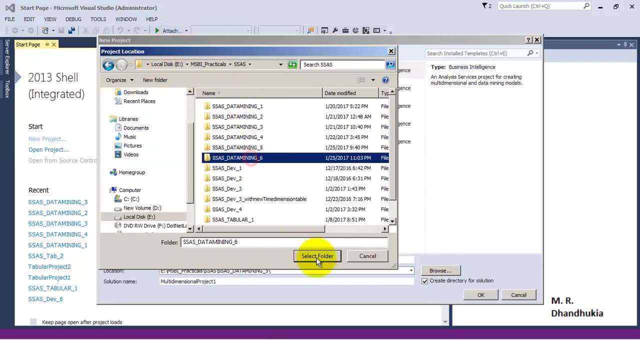 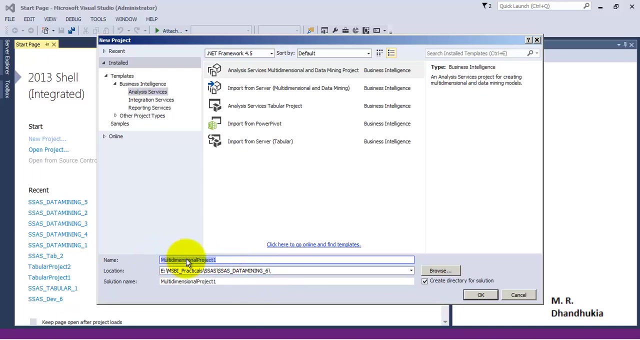 Hello friends, in this video tutorial let us see the algorithm of sequence clustering for data mining in SSAS. So for the purpose of this video tutorial, let us go and create a new project Now. let us name this project as SSAS Data Mining 6..